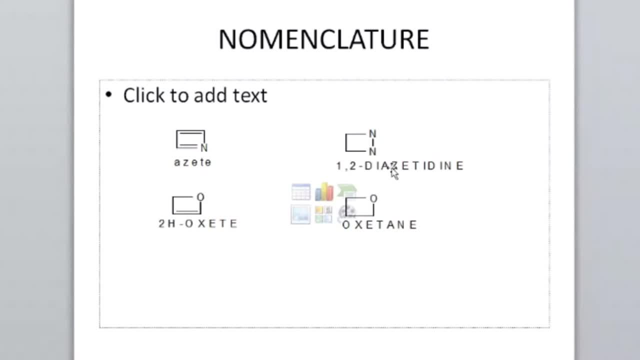 two. and because we have two nitrogens, die as a TD, die as a TD. the third one: you have oxygen, four membered ethereal cycle. one double bond for oxygen, because it is I the valent. you cannot have a double bond here. so for oxygen, four membered. 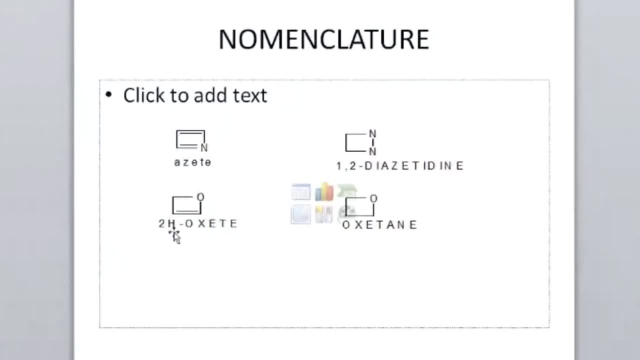 ethereal cycle. you can only have a maximum of one double bond and oxygen. when you're numbering, this is number one and then you move next to where there is sp3. oxygen is number. this is number two, number three, number four and since it is four membered, it is after there. this- it is four membered- must be here to H exit. 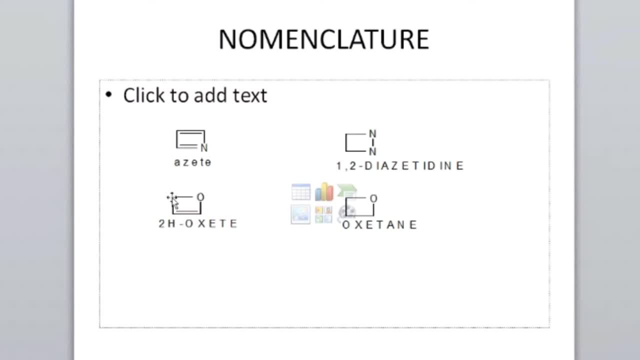 because the indicated hydrogen is at position two. here- please watch the video- is one true. always you make sure that they be headed. hydrogen has as low a number as possible. that's why you can start one, two, three, four, otherwise it would be 4-h. so the numbering is as that you read to first. so that's why it is to edge Opus. 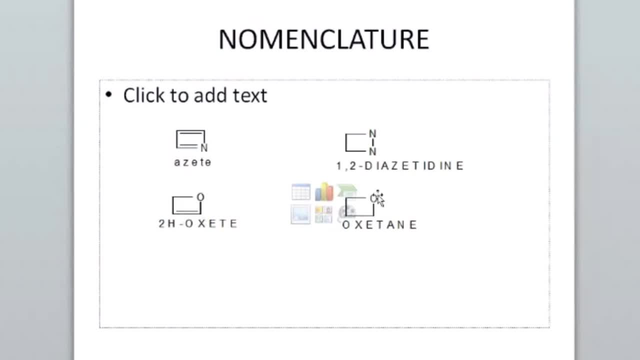 eat. the last one is an seule, which has one oxygen form-membered oxidation of you oxeton, again oxetine in thirty, plus oxygen constitution. actually, this is the second one, two following another one, two, and you know we will be- and using hydrogen also, the number one be applied to it again in transferring this: Zaragoza, Liam Stan and. 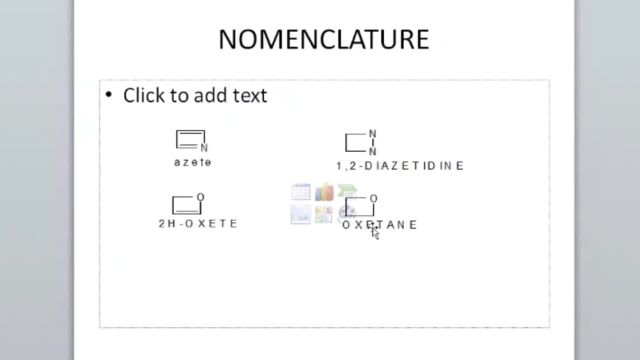 this example, the last time it is V nasa, we should. classic condition of ox, the ball which acts to another Royまた franc. Again, we said: eat for fully unsaturated and attain for fully saturated. Continuation of nomenclature. The first one: you have Oxygen and Nitrogen and in terms of priority, 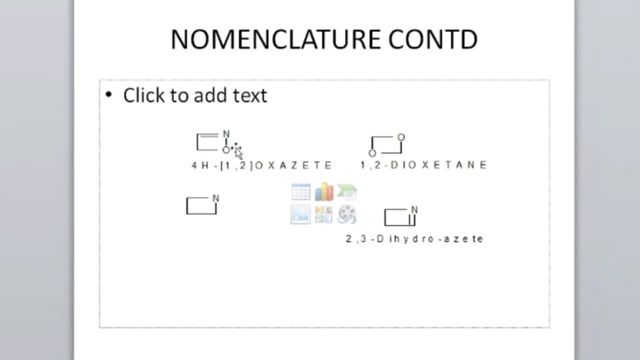 Oxygen comes first because it is in group six. at the top, The highest priority atom is Oxygen. you go down in group six, then next you go to group five, where you have Nitrogen, Phosphorus, ETC. 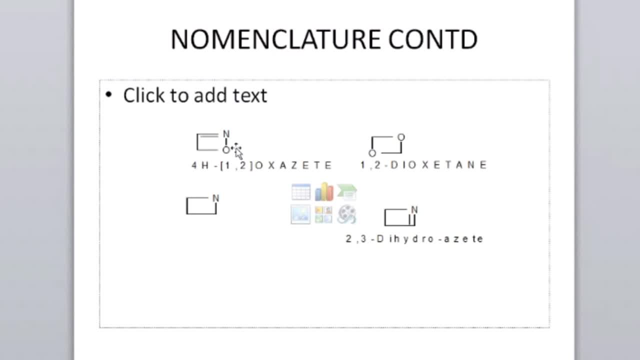 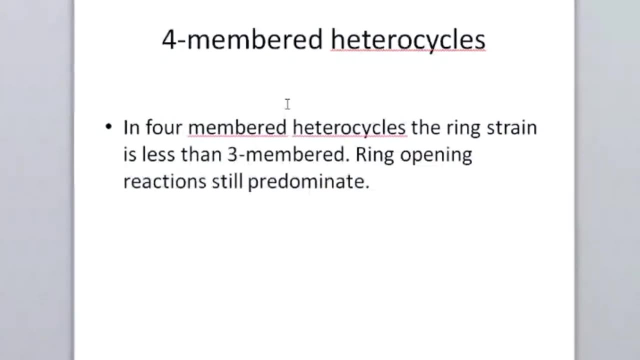 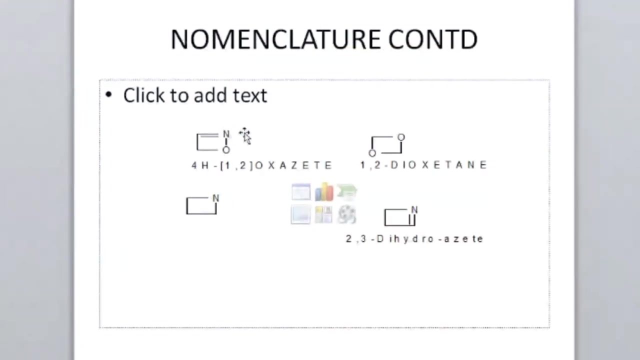 then you go to group four, where you have Silicon, and then you go to group three. So the numbering here will start from Oxygen. so this Oxygen is number one And this, So Oxygen is number one and this is number two, three, four. 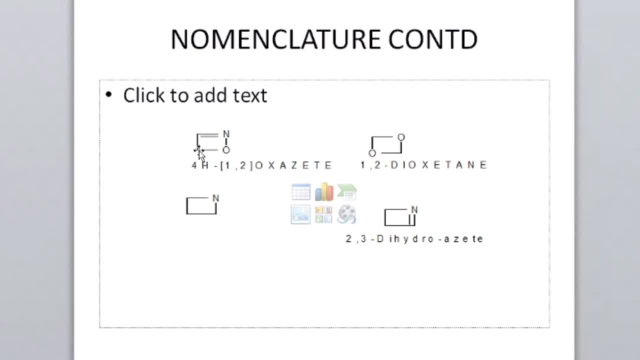 One, two, three, four. When you start from Oxygen you don't go this way. you go to Nitrogen. So Oxygen is at position one and Nitrogen is at position two. So that's why you write one, two, then Oxygen comes first. 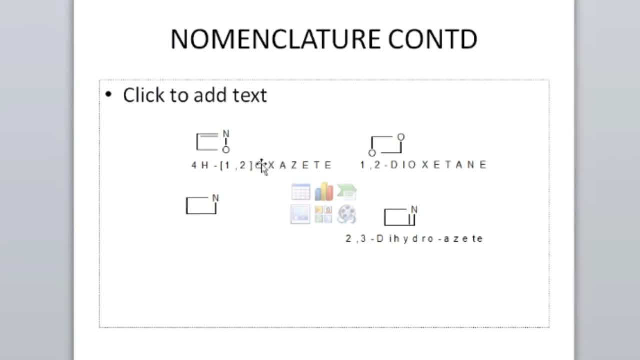 So it is like OXA and then AZIT, So OXAZIT, Because you can't say OXA, because it is followed by A, so one A goes. So that's why you find that is one, two OXAZIT. 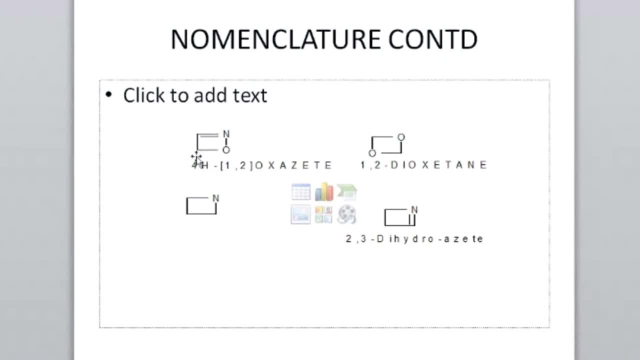 And then the four H indicates the position of the Hydrogen, which is SP3.. And the position of Hydrogen, which is SP3, is here Here. So this is one, two, three, then four, So that's why it is four H. 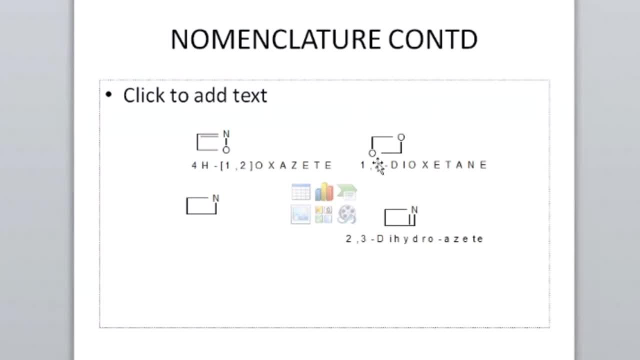 And the next one: four membered with two Oxygens- The name. So I said that these four membered, it will cycle. The nomenclature is wrong. It is supposed to be one, Three, Because when you start numbering from here, this is one, this is two, three. 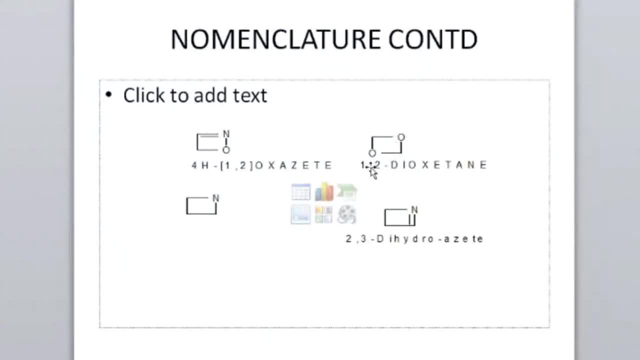 So it is supposed to be one three, So. So, once you get the notes- because it is something that can be corrected- you write one three and then DIOXETINE, Because it is fully saturated. Then the third one on this slide is four membered with Nitrogen. 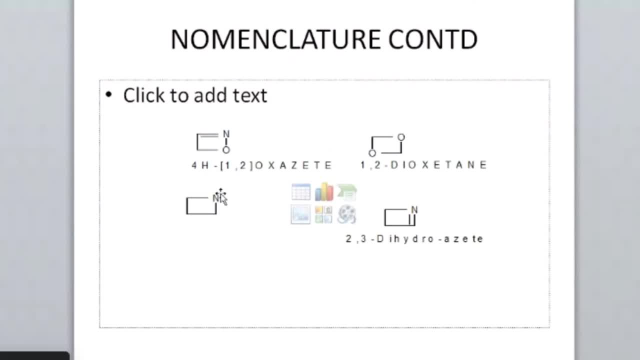 Again, one Hydrogen is missing, But there is no problem, because these are shorthand, So this is called AZETIDINE. The name is not there, But you can write somewhere that it is AZETIDINE, AZETIDINE. 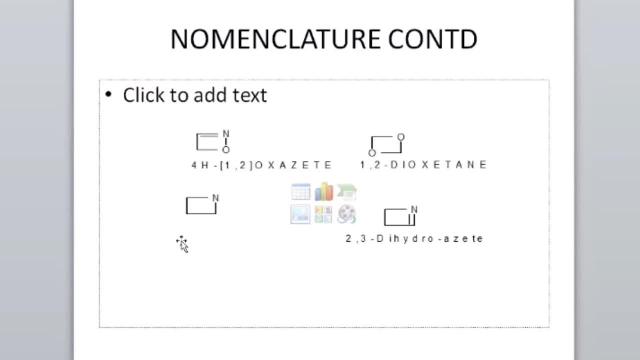 Or AZETANE. So this one is AZETIDINE, You can write it somewhere- Or AZETANE. And again, Most of this, Because you don't have a chem draw. I am the only one who can do the correction. 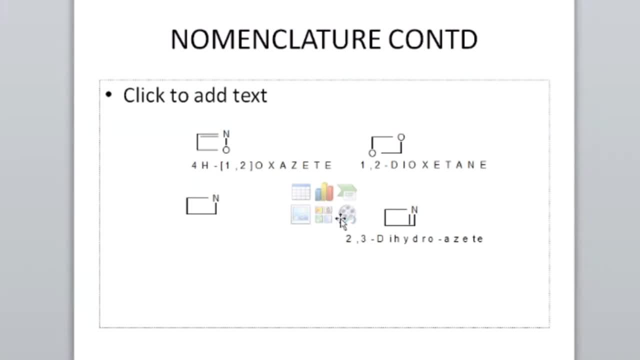 So I'll do it and send you the corrected one And then the fourth. The fourth, it will cycle. Yes, the fourth it will cycle is here. This thing keeps on jumping. So the fourth it will cycle, which is here, has Nitrogen and one double bond. 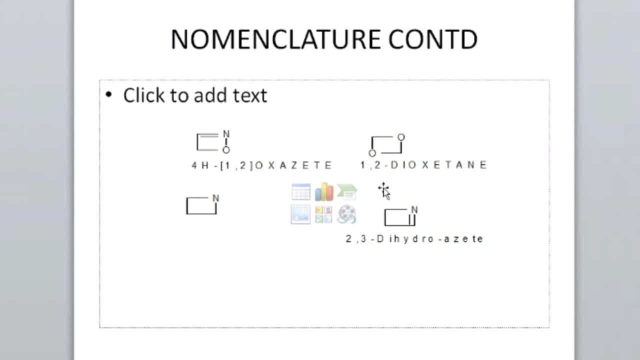 But we said that for Nitrogen to be present in a four membered, it will cycle. The maximum number of double bonds should be two And therefore there is also another double bond here. There is a double bond here. There is a possibility of having another double bond here. 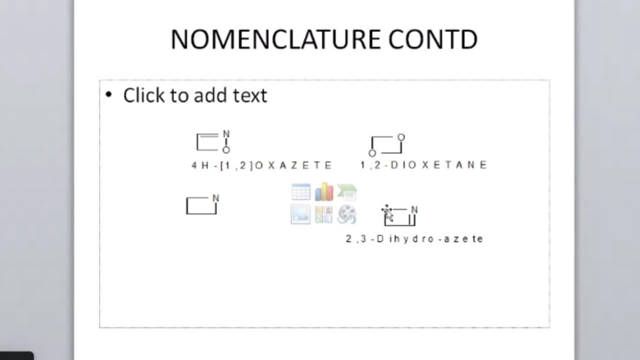 But it is not there, Which means that this double bond was Hydrogenated And when it was Hydrogenated. so you added a Hydrogen here and added another Hydrogen there, And because of that we say that you have added two Hydrogens. 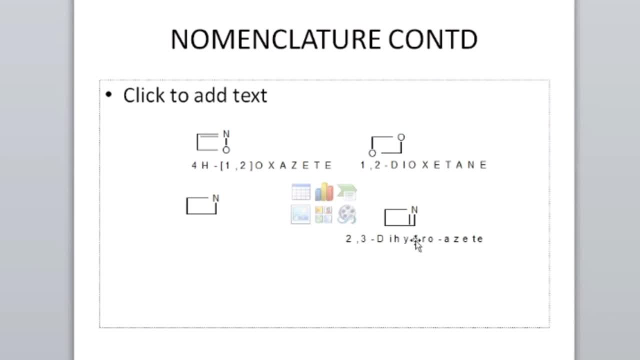 And that's why you have dihydro, That you have added two Hydrogens at positions two and three. So if this is position one, If this is position one, This is position two And this is position three. So when numbering this, one, two, three, 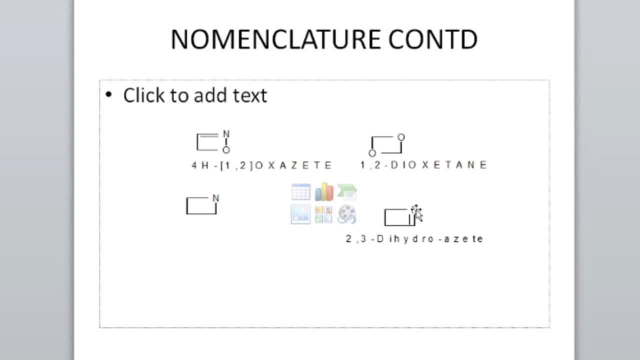 Again, you number in such a way that You go towards the SP3s. See, they are here. So this is one, two, three. So the Hydrogens were added at positions two and three. That's why it is The nomenclature is two, three, dihydro.